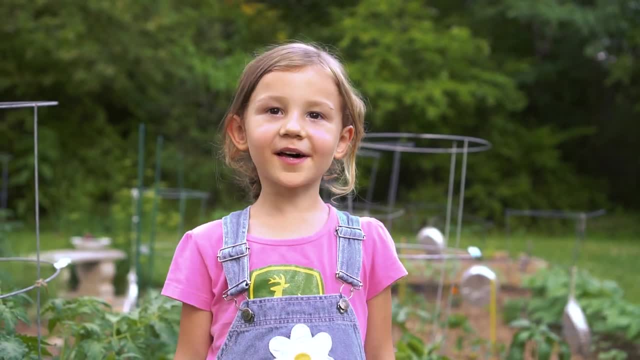 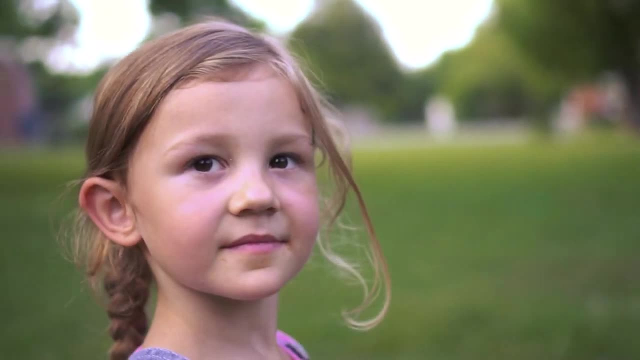 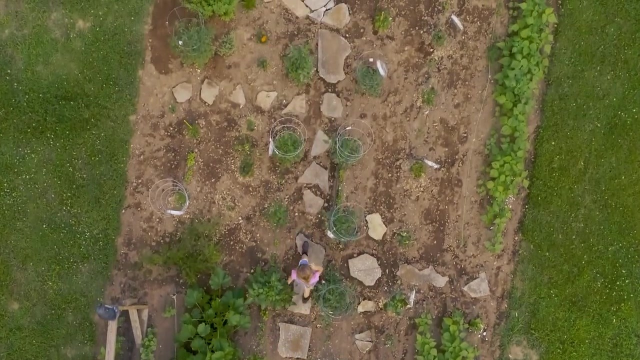 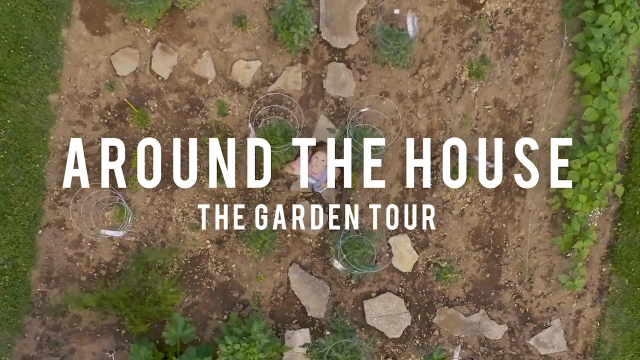 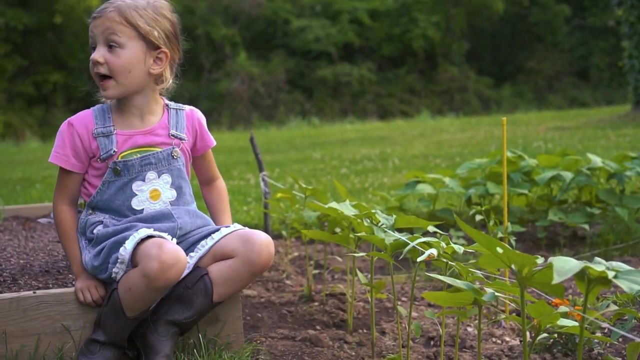 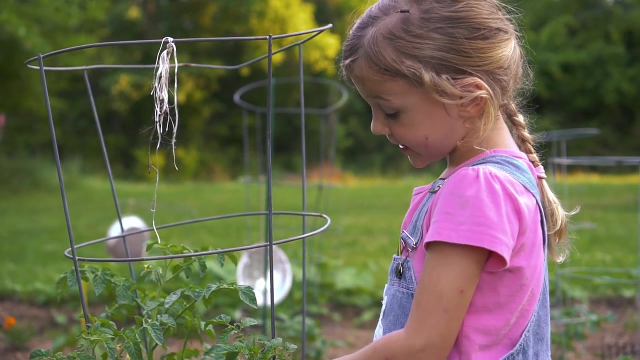 Hi, my name is Rachel. This is my gardening show And now it's time to start. So these are sunflower seeds. They have beautiful sunflowers, And let me show you some other plants that we got here. Come on, This is a cherry tomato plant, And you see, these flowers, They are cherry tomatoes. They're. 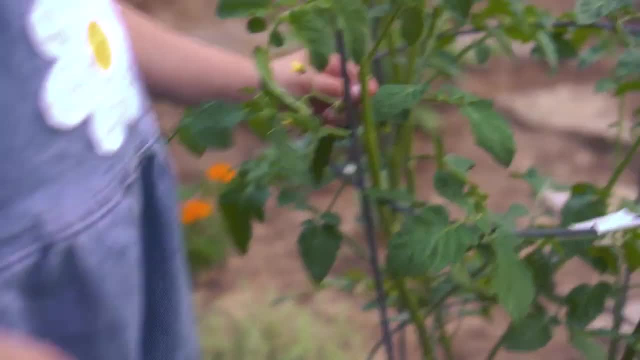 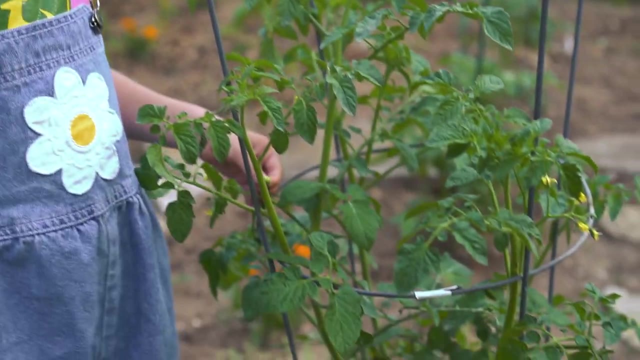 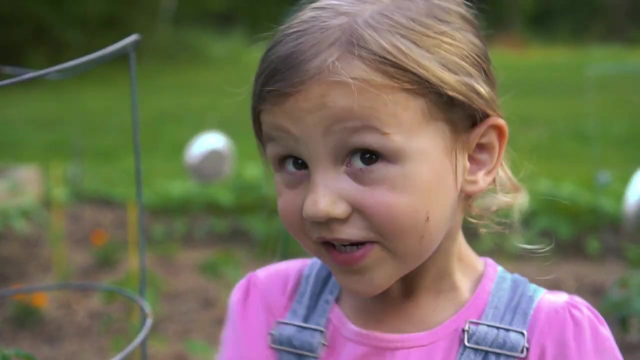 my favorite tomatoes. So, yes, Do you see this? That is a baby tomato. But yes, all these flowers in this baby tomato are cherry tomatoes. They're the best. It's just because they're sugary and sweet, They're the best. So you kids have fun with those tomatoes. But one. 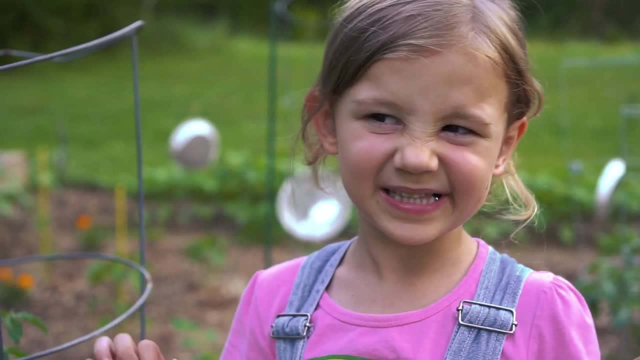 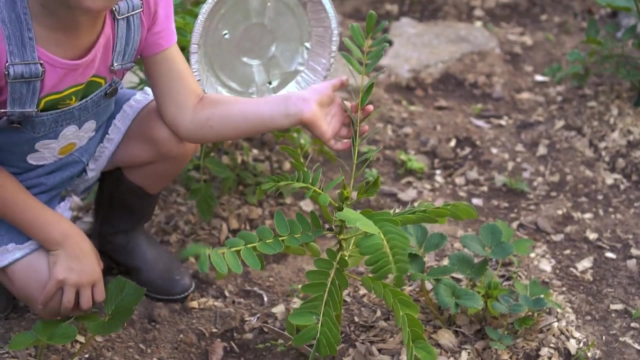 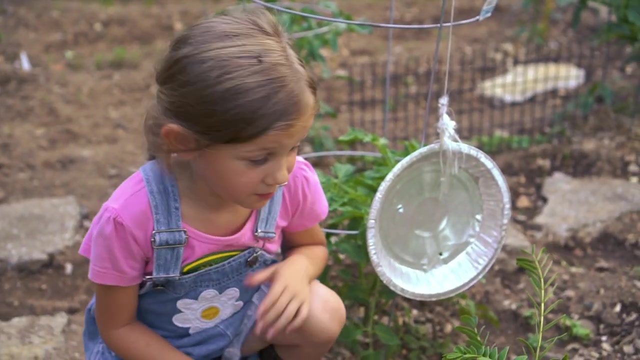 second, Remember to pull this down if you don't like that part, But remember when they're all red they taste better. This popcorn plant: if you rub the leaves and then smell it, it smells like popcorn. They have pretty yellow flowers that look. 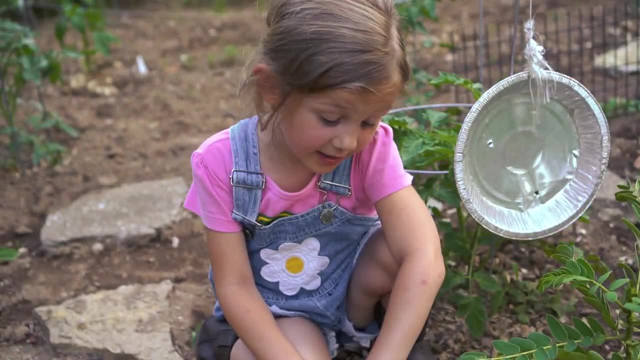 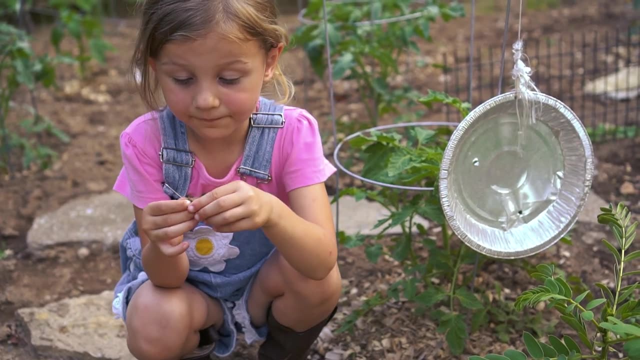 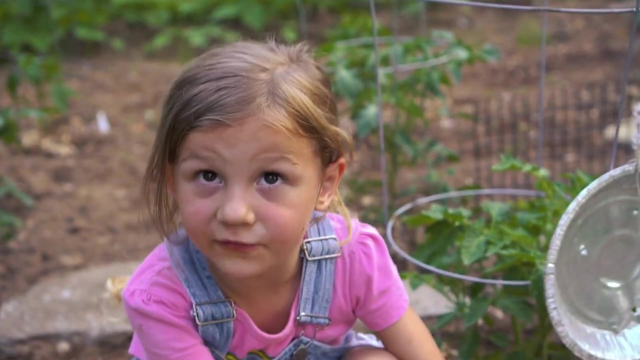 like popcorn. These are strawberry plants and they grow and you put baggies over them, so the bunnies don't get them. Wait until they're. the more redder they get, the more fresher they get. So if you want them real fresh, you gotta leave them red for a couple. 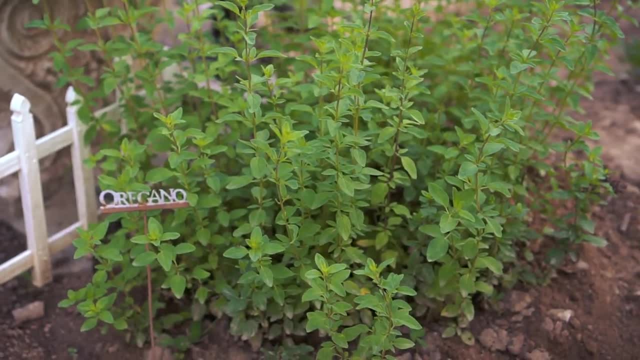 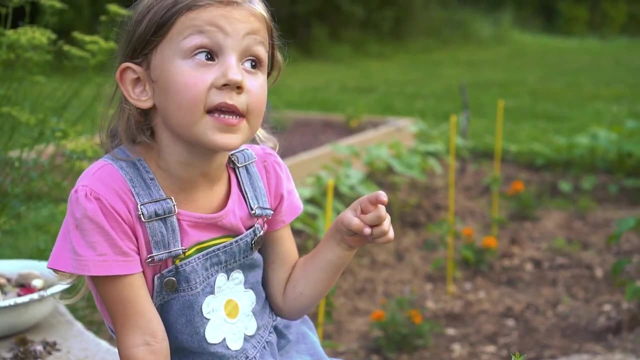 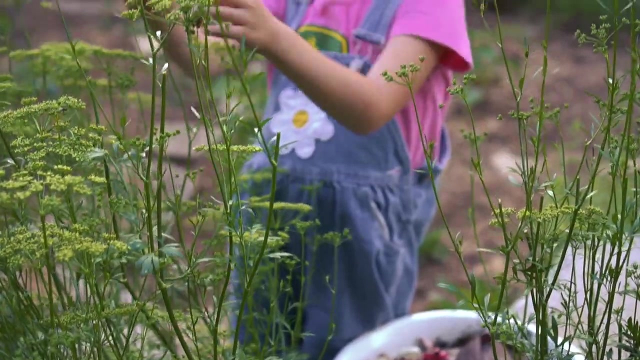 days and then they'll be tasty. So this is oregano, and if you rub your hands through it, it smells wonderful And it's good for sickness. I heard This is another herb that is delicious. What herb is it? I don't know. 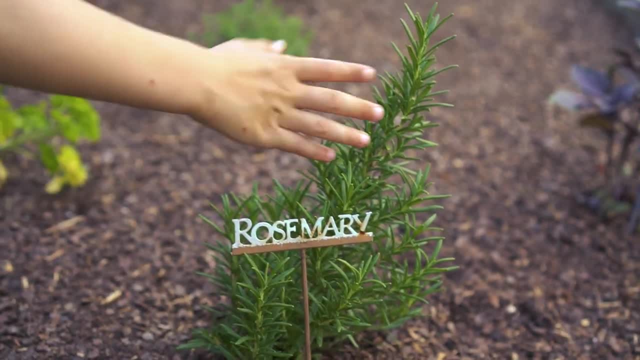 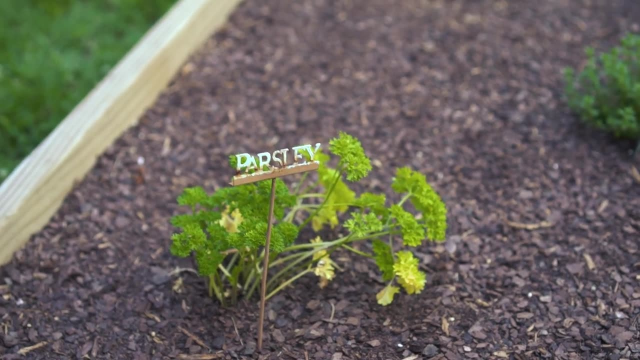 This is a herb box. Yes, What is it? Yes, and if you put your hand on it and rub it, it smells wonderful. This is parsley, and let's see what else we got. This is purple basil, and it's the best. 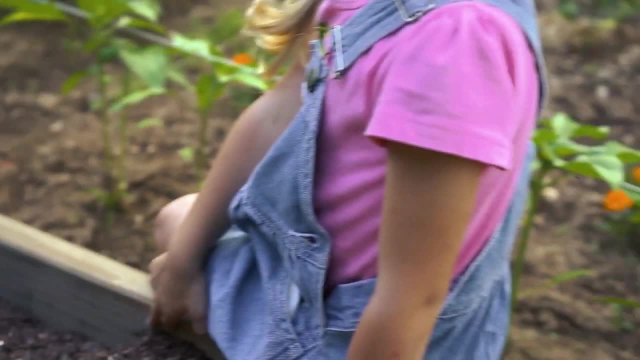 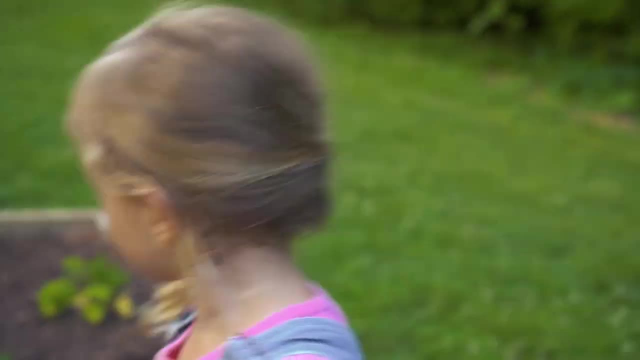 Do you see that leaf that's broken? You might have to put some bug spray on that Thyme- this is thyme. This is lemon balm. This one is some mint. This is a jalapeno plant. It's really good.